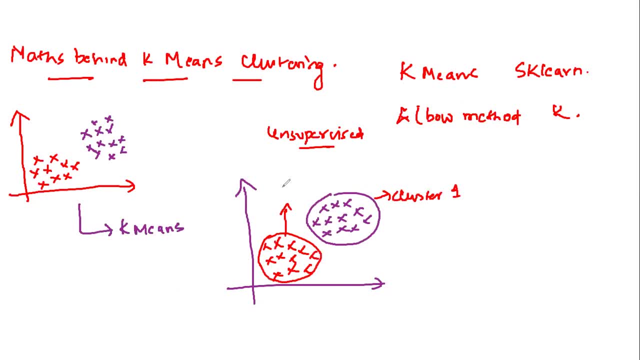 So I can call this as my cluster one and this is my cluster two, And that is the thing that K-means will be doing. But to do this, we are going to discuss first of all what is the algorithm that is basically used. 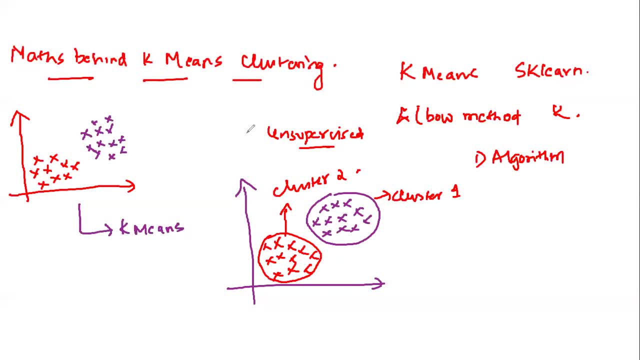 There are five steps of algorithm that we are going to use and to actually define my K-means clustering model. The second thing is that what metrics we'll be using. There are two metrics that we use in this. One is Euclidean distance and 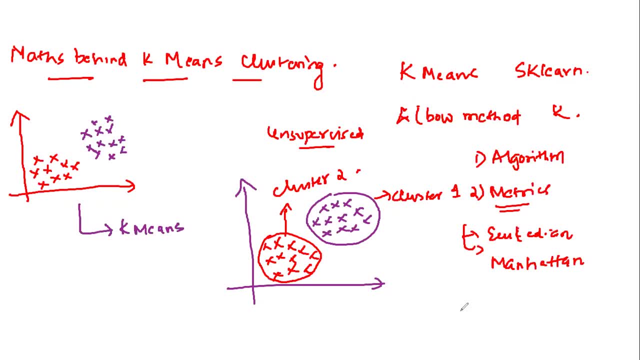 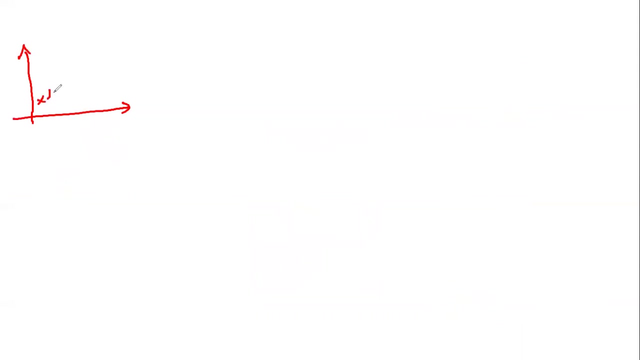 one is Manhattan distance. We'll be discussing that. Then the third topic that we'll be discussing is something called as what is ELBO method. This ELBO method will be used for selecting the right, selecting the K value. So let us go ahead and start the discussion Now. suppose I have a point. Okay, so I have some points like this: 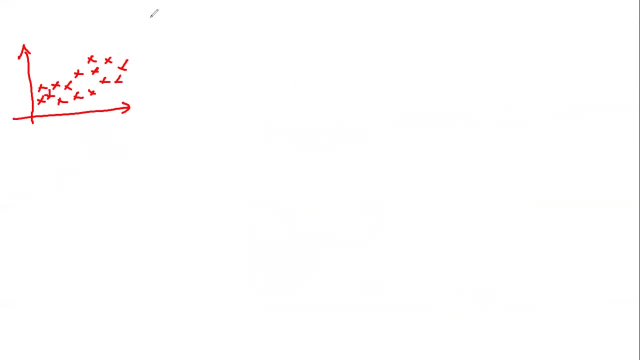 Okay, so what does this particular K-means clustering? What are the steps in this K-means clustering? So first step says that we have to select the K value. This K value are nothing but centroids. I'll explain you what is centroids. Just give me a second. 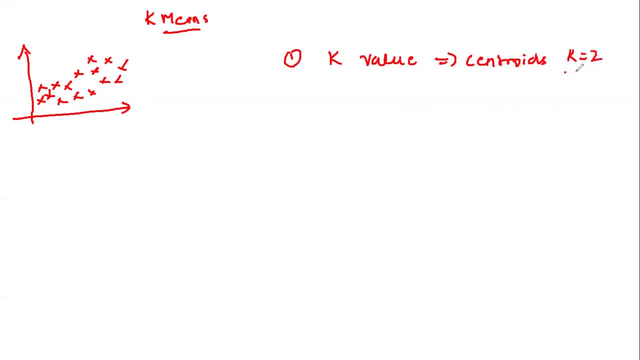 Suppose I consider my K value is 2, and I'll also show you how we can select this K value, How I am selecting it as 2 whenever I have this kind of distribution. Okay, by just finding the similarity between the data, how can I group them and what should be my K value? 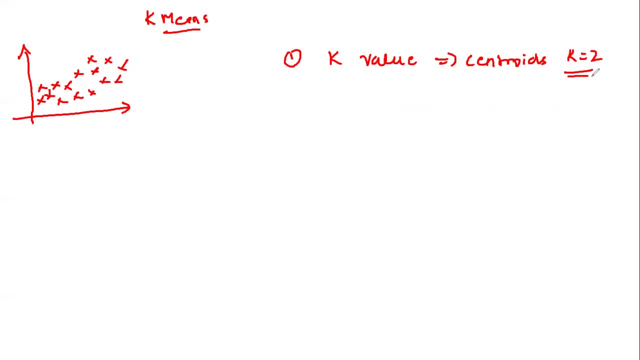 How many centroids should I be having? If I have two centroids, that basically means two clusters, And I'll show you how to select the K value in a while. The second step that we will be doing is basically we need to initialize these two centroids randomly. 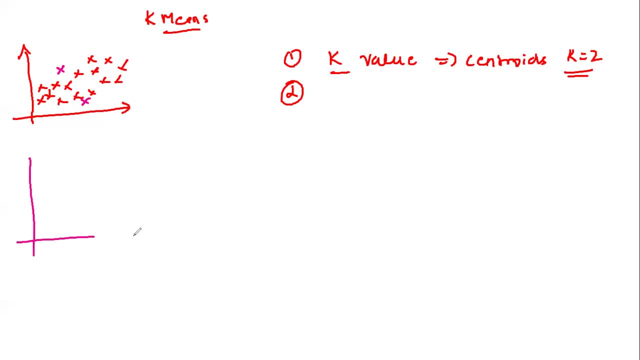 Suppose, if I initialize these two centroids randomly in this plane, then my data will look something like this. Let me just draw the point once again. So these are my points Right, and, as I said, that I'm going to initialize my two centroids randomly. 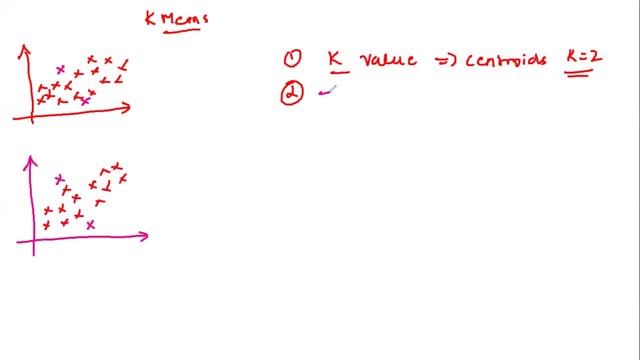 So I have initialized one centroid and one centroid only. So initialize the centroid, Initialize the centroid randomly In the plain Okay. initializing means that I'm just initializing some points over here. The next step is basically: I need to find out the distance. 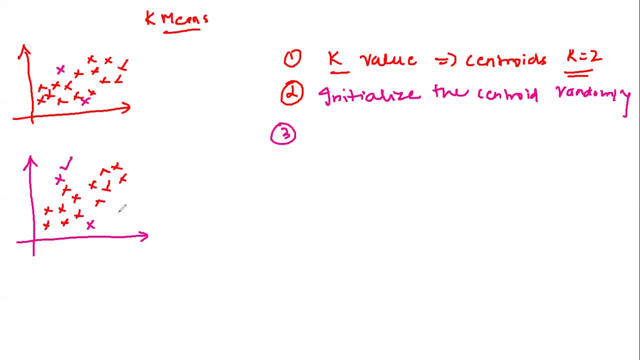 which are my points that are nearer to this particular centroid and which are my point that are nearer to this particular centroid. So, for this, what I'll do is that I'll make this as blue color. Okay, so, in order to find the distance, 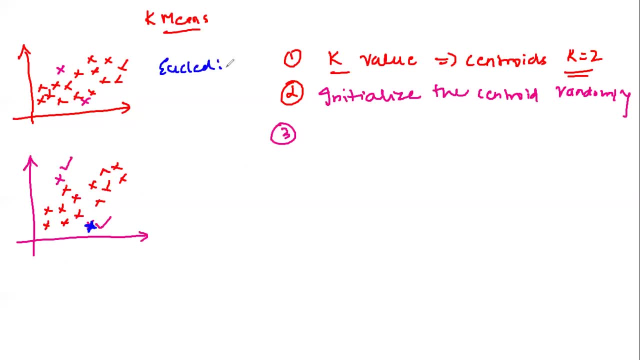 here we are going to use a Euclidean distance, which is called, as you know. if we use a Euclidean distance distance, we will be able to find the distance which are the points that are nearer to the blue points and which are the point that are nearer to the pink. 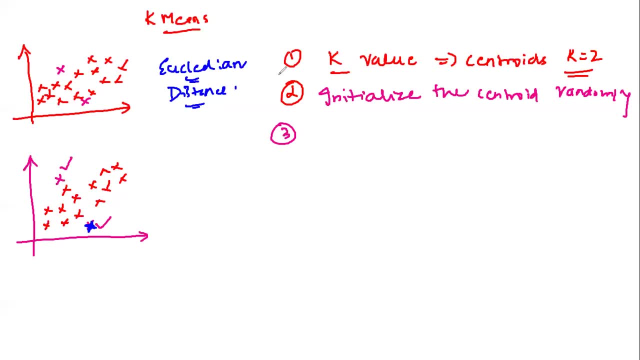 points. in order to draw it, you can just use a simple technique. okay, I'll just draw our two lines over here. one straight line I'll draw like this. the other straight line that I'll draw is like this: now, when I draw this, whatever points I'm coming on top of this particular straight line that will 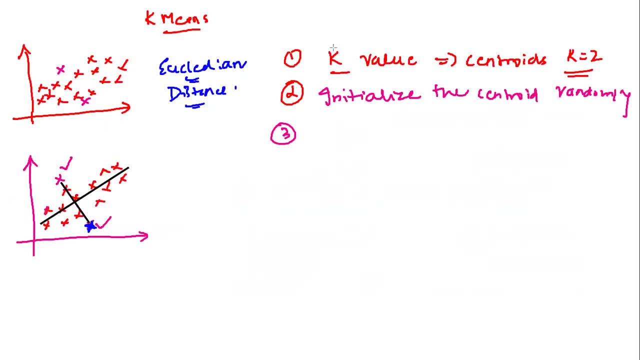 become my pink. let me just draw this particular thing once again. so this will become my pink color. that basically means that this is basically nearer to my pink points, right, and similarly this blue point, this: whatever points are present below this particular line, it becomes my blue points. so here you have all the blue points now. by this we have categorized. 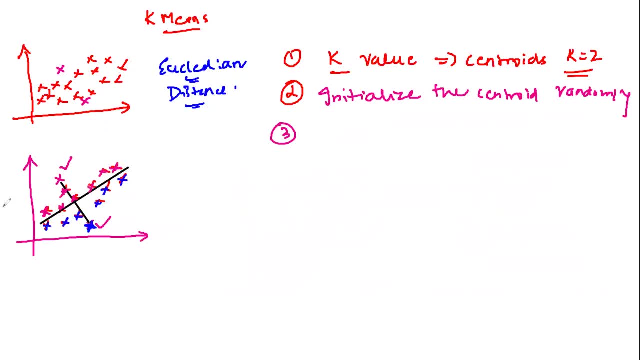 two group of data, but still the step is not done. right. then what we will do is that you select the group, we select the groups right, we select the group and find the mean value, and find the mean value right. so when I, when I take this, when I take, 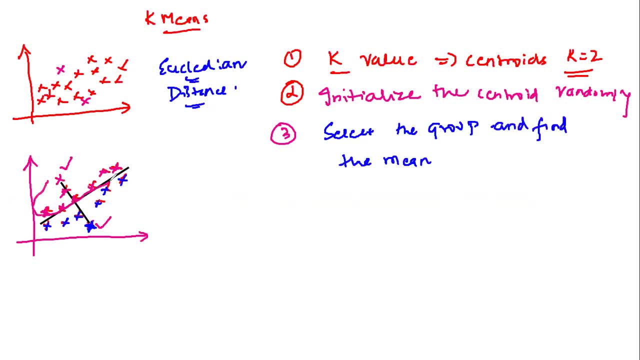 this, this pink color group. you know, I'll find the sum of all this particular elements. I'll find the sum of all this particular elements. similarly, for this blue statements also, what I'll do is I'll find the sum of. so when I say sum, basically, I'll find the average of all these elements. okay, average, very important. 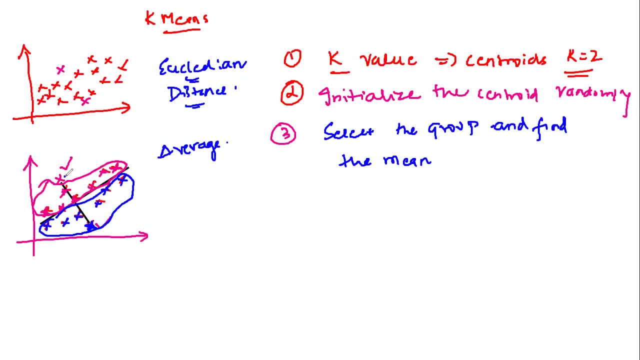 after I find the average of the spring points, I have to move this centroid to that position. similarly, I have to move the centroid for this particular position based on the mean value that I get. so what I'll do is that, after this and again, draw a straight line now how my data will look like. so my new centroid: 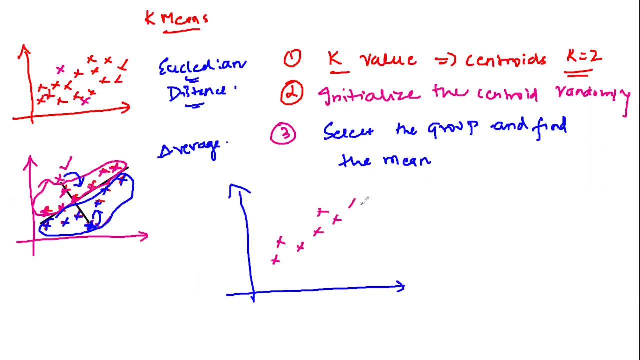 suppose this is my pink point right, and suppose my new centroid position is this one- okay, after I moved it from here to here. similarly, my blue position will be somewhere here. okay, and then I'll be having all my blue points now. after this, what will happen is that 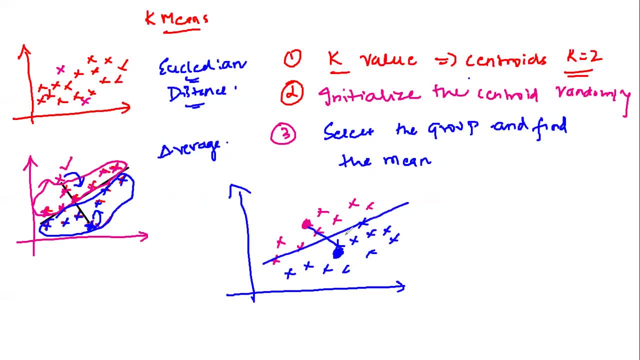 again. I'll create a straight line and perpendicular like this, you know, to find out whether any points has been moved or not. now i'll i'll repeat this whole step, that is, from the second one: initialize the centroid. now. i have now what you know. i have updated my centroid and moved the position, so i have to again, you know. 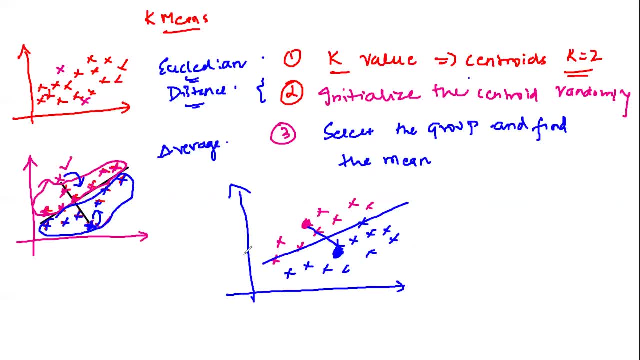 find out which all points are nearer to the point again to test. when i do that, you can see that some of the pink points have moved towards blue. so this will become my blue pointer, and this blue point will somewhere become like a pink. okay, suppose it becomes a pink one, right? then again, what will? 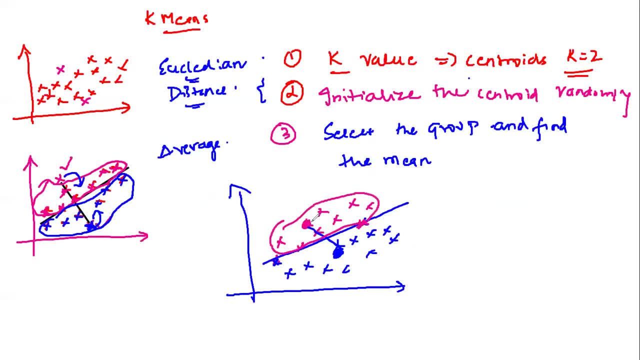 happen again. i'm having two groups. again, the mean will be calculated. my centroid will be updated to this particular position. similarly, this particular group will be calculated again. my this position will be moved over here. my blue point will be moved over here. now, this step will happen again. 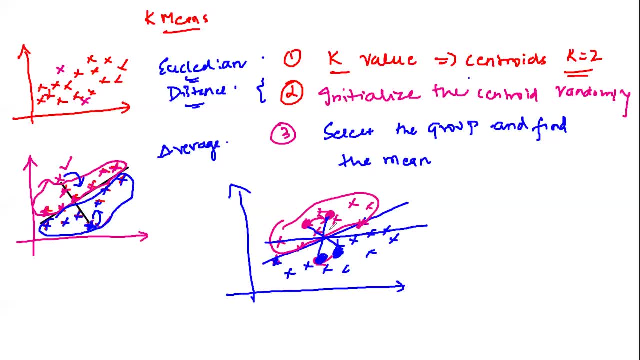 i'll go and try to find out the center elements. and finally, you'll be thinking that this step will be happening unless and until we get a fixed number of groups. okay, and no point movement will get changed. so that is my final step, as soon as i'll be able to do that. that basically means that it is giving me two clusters and these: 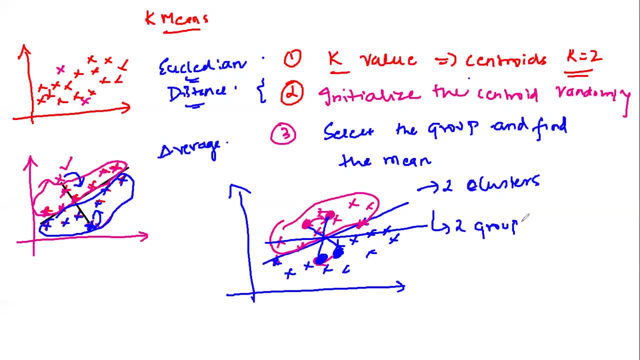 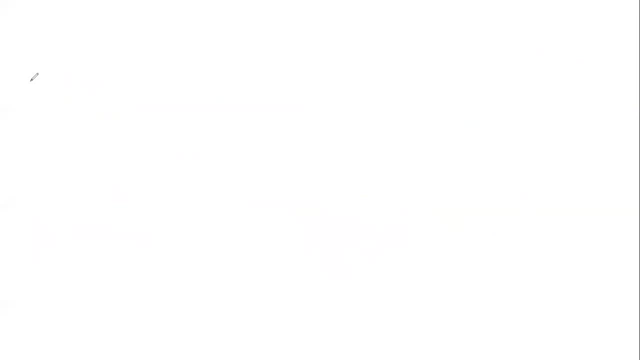 two clusters are nothing but two groups. right, and this is because i'm taking the k value as two. okay, but i have not told you how i am selecting the k value as two, why i am selecting the k value as two. so again to begin with. guys, see this and just draw all the diagrams one by one now. 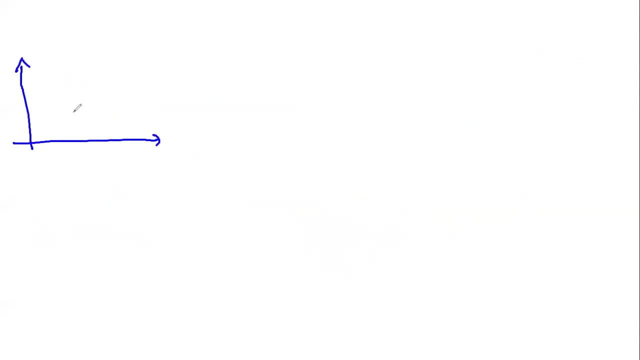 okay, so initially this is my position. okay, so initially my points were in black color, suppose. okay, now i wanted to implement a k-means clustering- okay, in such a way that i need to group these two data and, as i told that, my next step was basically to initialize centroids. initially, this is one. 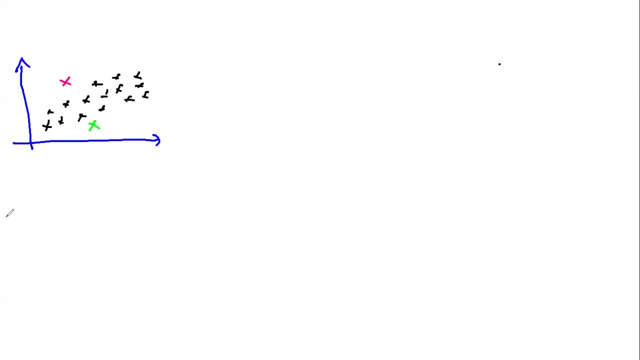 centroid, and this is one centroid, suppose. then, after that, what i did is that i created a straight line, i divided this point. this all became pink color, right, because these were the points nearer to the pink color, and now these were the points that became nearer to the green. so now i 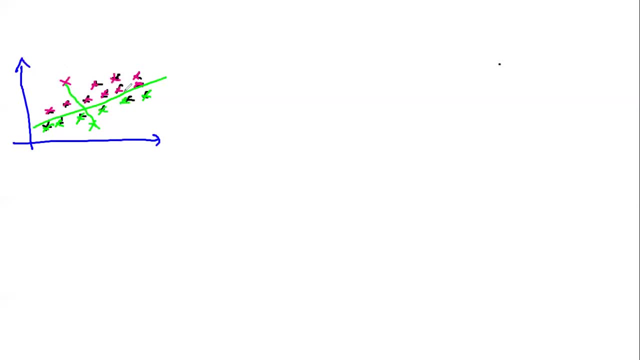 have two centroids. now what will happen is that i'll compute the mean of all these points and i'll update my point based on that particular mean. this is my centroid, so i'll update that in my next graph. what will happen is that i'll draw the next point. 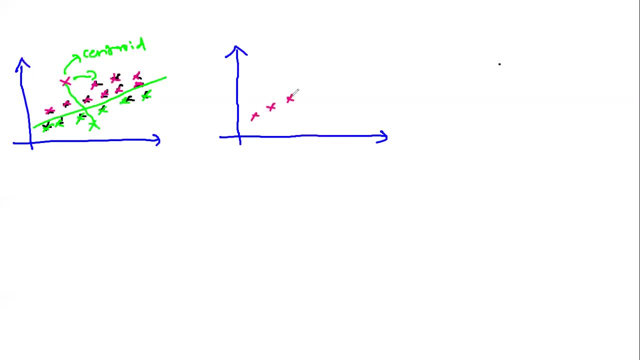 i'll draw all the pink point as it is okay, but my center point has now been updated to this particular point based on the mean of this value. similarly, with respect to my green, my green will also get updated somewhere over here, right, because i'll find the mean. 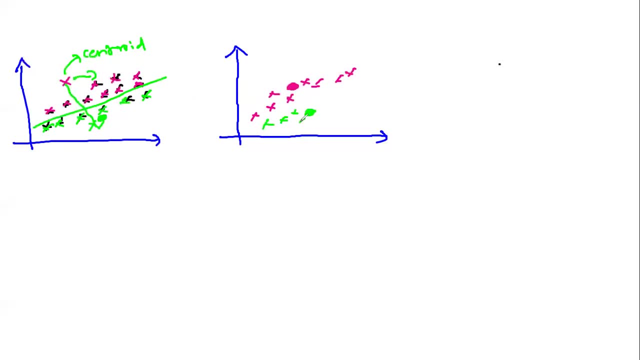 suppose my green has come over here. my centroid and all the points are there now. this talk will be processed unless and until we get exact number of clusters based on the k value that i have, such that no movement of points are happening between pink and green, and once it is done we can say that our model is ready. 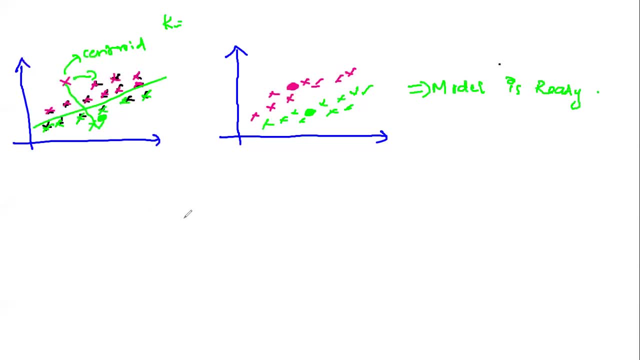 our model is ready and it is able to do the classification. now, as discussed, that how i am computing the distance, i will be calling that as an euclidean distance. the euclidean distance basically says that if i have a point, p1, p2, p1 is represented by x1 comma y1. p2 is represented by x2 comma y2. 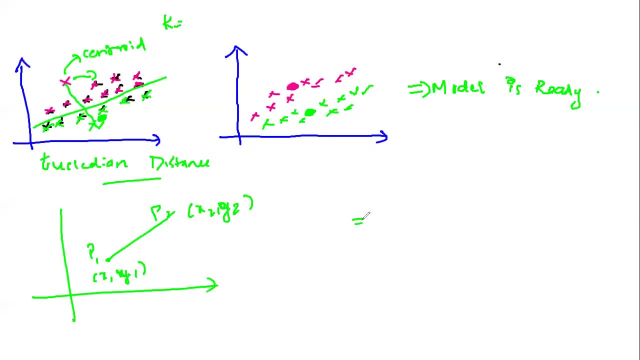 then euclidean distance, that is, the distance between these two point, is basically given by root of x2 minus x1, divided by y2 minus y1, whole square plus right? so this is basically my formula. okay, so this is how euclidean distance is done. now the next thing is that: how should i select? 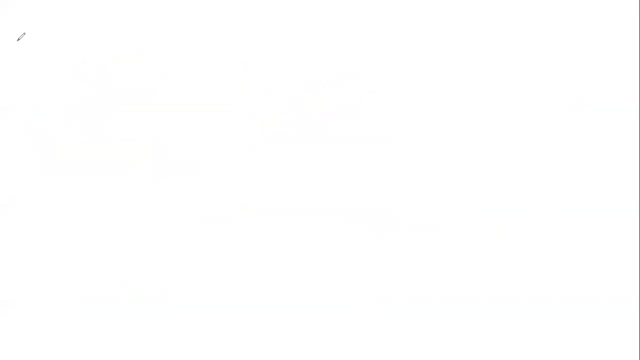 my k value. for selecting the k value, we basically have something called as elbow method. now elbow method basically says that i will be running a loop from k is equal to 1 to 20, suppose. okay, in k is equal to 1 to 20. that basically when my centroid is 1, suppose. now, this is my point. 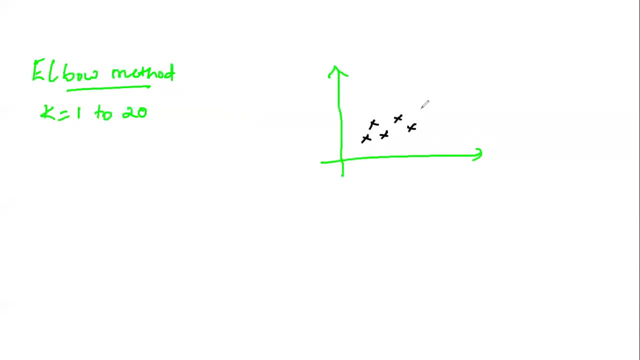 okay, and i'm just drawing all the points like this: so for k is equal to 1, i'll be running the whole process of k means. so that basically means that my point will get initialized somewhere here: for k is equal to 1.. then what i'll do is that i'll find out the distance. that is w wcss, which is nothing but. 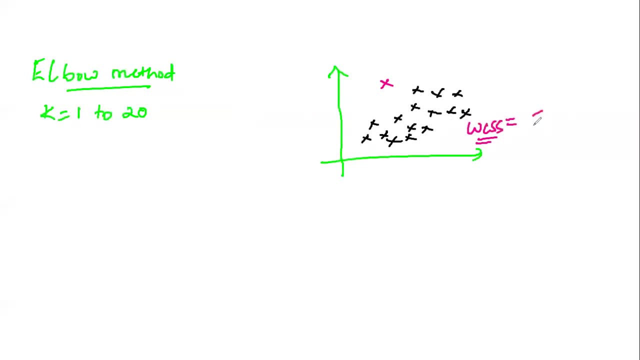 within cluster sum of square. okay, and this is basically given by summation of i is equal to 1 to n, the distance between the, you know centroid plus all the points. so i can write c of i plus x of i, whole square. so i'll calculate the distance between all these points. 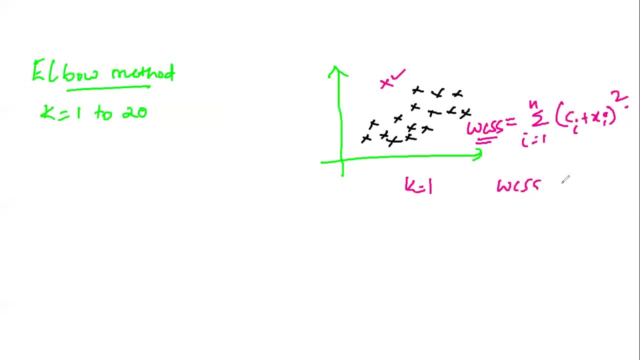 and for the initial, even the case one, our wcs's value will be very, very high. so when i just go and plot my diagram with respect to k value and with respect to wcss value, initially, when my k value is 1, my wcss value will be also high. then, with k is equal to 2. 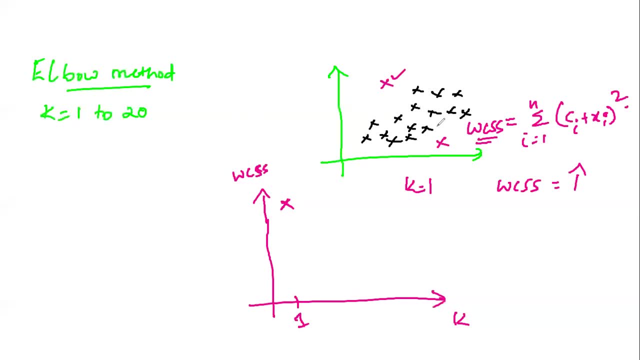 now, when i have k is equal to 2, i'll be having two centroids and i'll be computing the distance for the point that belongs nearer to this particular value. so this will be my distance: 1 right, all the distance to this point and all the distance. 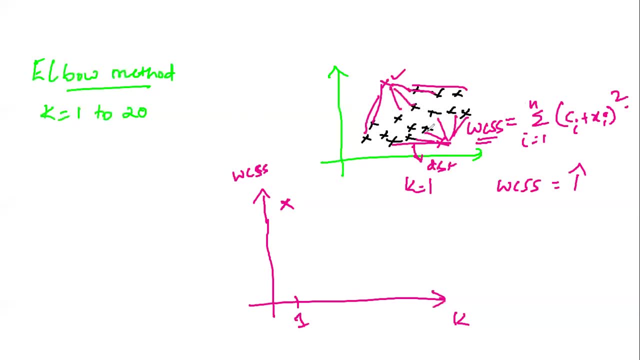 to this point. so i'll calculate the sum. okay, i'll calculate the sum and, uh, after calculating the sum, i'll be getting all the values right. so now, for k is equal to 2. what will happen is that this wcss value will obviously decrease, because now i have two centroid. similarly, when i increase, 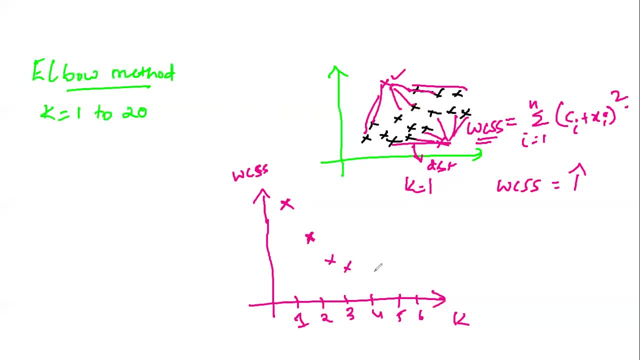 my k value, my point, will be getting decreased, but at at a certain point it will become normal. normalized it will be become. it will be working in a very slow manner. so how do i select this k value from this elbow method? and this is basically called as elbow. 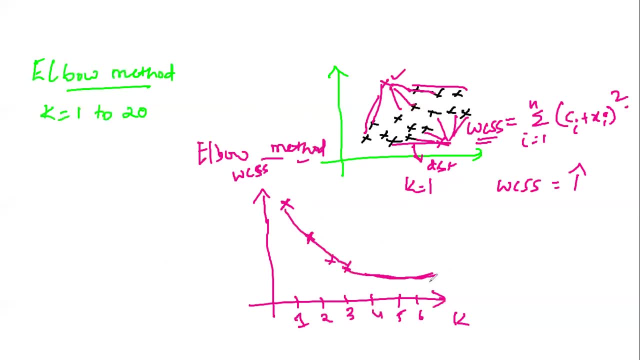 method, guys. this elbow method is white is called because it is in the shape of elbow, our elbow. again, i have shown you this in the practical part, guys. what i'm going to do is that once you complete this theoretical explanation, you just have to go and follow that particular practical part. now, at this point, how, which value we have to select. we.